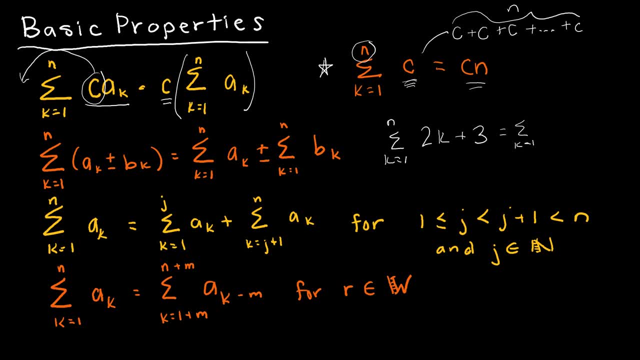 into the summation as k goes from 1 to n of 2k, which of course I could use that property and put the 2 on the outside and say 2 times the summation of k and then I could add to that. 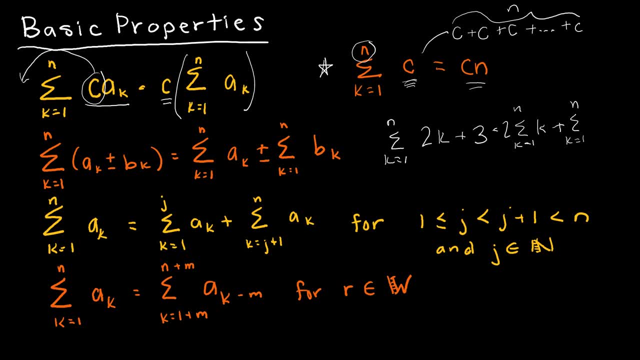 the summation as k goes from 1 to n of 3, where I would obviously be using this property. The next property says: if I have the summation of some sequence, I can split this into two parts, as long as those two parts cover the entire limit. 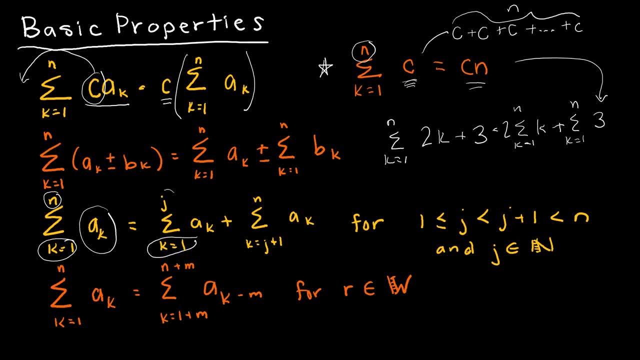 from lower limit to upper limit. So here, if I start at 1 and go to some integer j and then in my next one I go from the very next integer up to n, That's all this is saying is: hey, you're going from your lower limit. in this case, my lower limit was 1,. 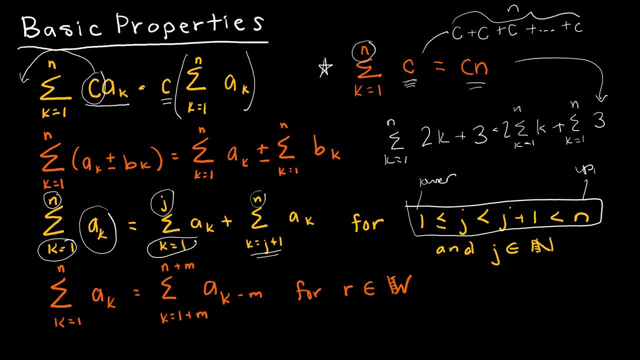 but it wouldn't have to be 1, so lower limit to upper limit and j between those two values, and obviously J plus 1 is between those two values. The last one is deceptively complicated, but it's something that you might use from. 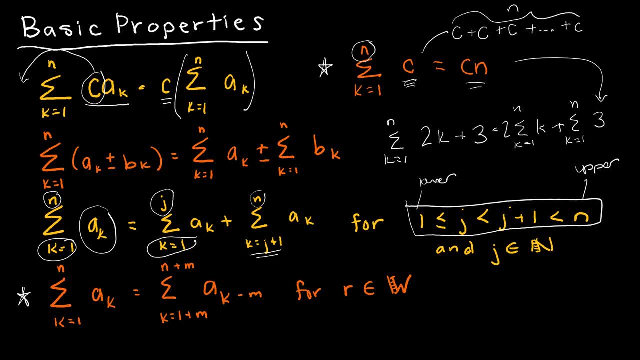 time to time, because, as we go through some of the formula in the next couple of slides, you'll find that some of the formulas start at 0 and some of the formulas start at 1, and so it might be that I have to add or subtract some. 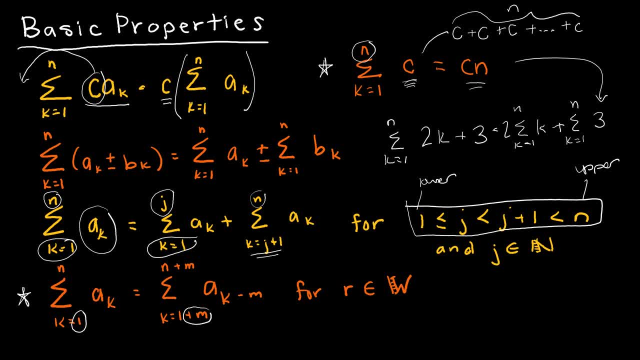 value from this lower limit of integration to make it equal 0 or 1.. So I can add M or subtract M. I've just shown addition. I can add the same value to each of those limits of integration, but then I'm going to have to subtract the. 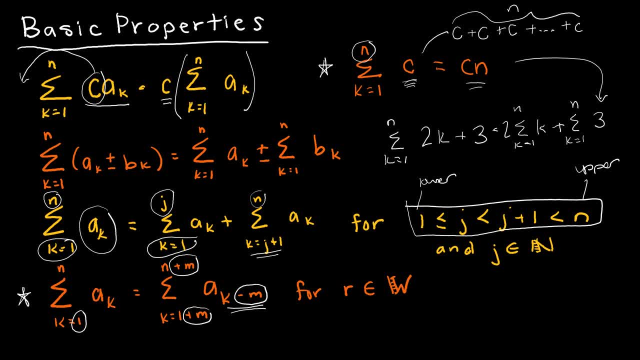 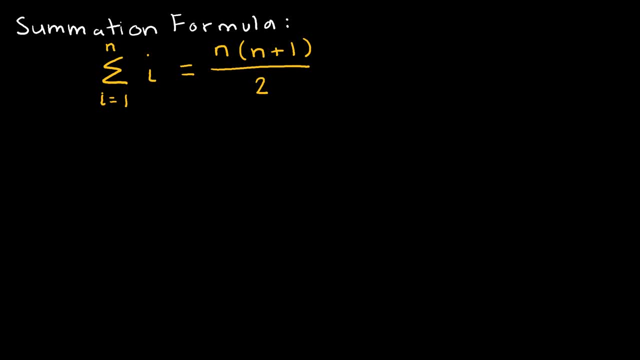 value here. So let's take a look at our first summation formula that says: if I want to find the sum of as i goes from 1 to n of i, then all I have to do is take n times n plus 1 divided by 2.. So let's. 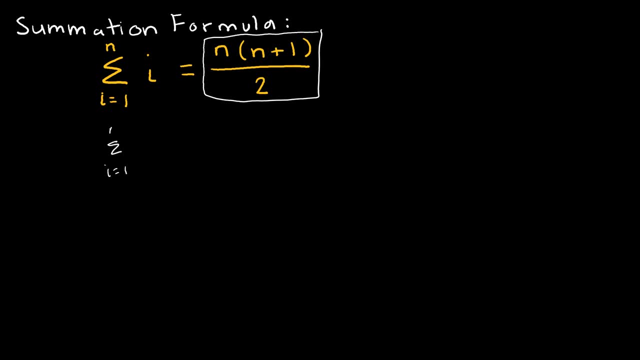 just look at a practice where let's say n is 7.. If n is 7 of i, then that's saying, start at 1 and continue to increase by 1 all the way up until you get to our upper limit, which in this case is 7.. Now I can easily add this in my 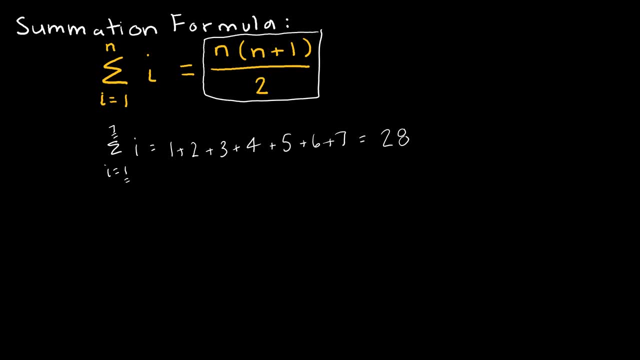 head or using a calculator to find that the sum is 28. but of course the summation formula comes into play when I can't just find it by hand, If I need to actually use the formula, or quite often we're going to use these formula in. 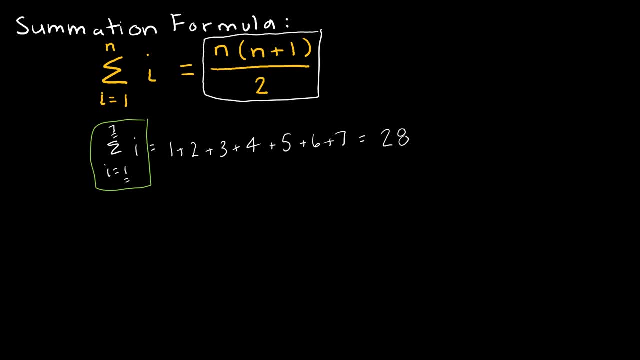 proofs, and so, of course, the formula is important. Now let's take a look at the formula and why it works. I'm going to add 1 through 7 again, so I'm going to add it twice, and the second time I add it, I'm just going to add it in the 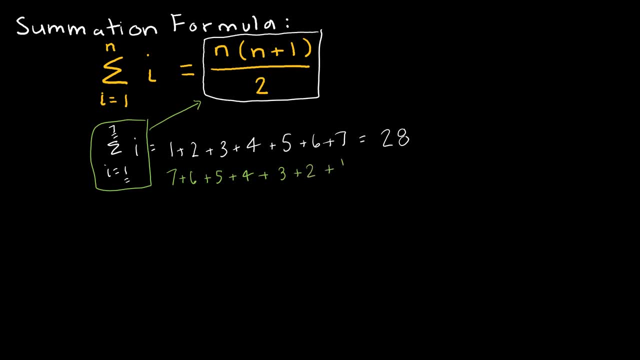 opposite order that I added the first time, which, of course, as we know, is going to still give me 28.. What happens is if I then add 1 and 7 and 2 and 6 and 3 and 5 and 4 and 4, and I continue, I'm just going to get a bunch of eights. and how? 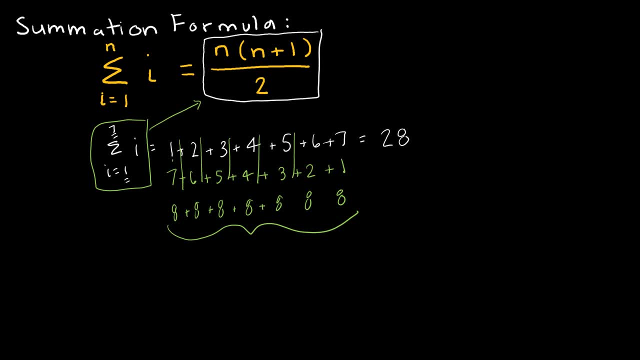 many eights am I going to get to add together? Well, I'm going to get seven of them, And what happens is then I'm taking 7 eighths added together, which I could rewrite as 7 times 8, and then, because I've added it twice, I just have to. 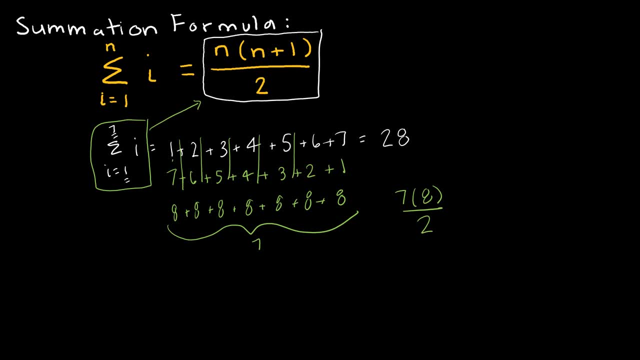 divide by 2, because I've found twice the sum, so I have to divide it by 2.. That's all this formula is telling me. So this formula says: as I goes from 1 to 7 of i, I'm going to take n, which is 7 times n plus 1. 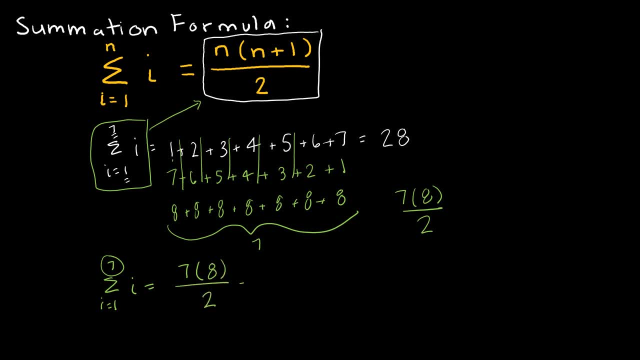 is 7 plus 1, or 8,, and I'm going to divide it by 2,, which is 56, divided by 2,, which is 28.. So we get the same value whether we're using the sum written by hand or using the formula. 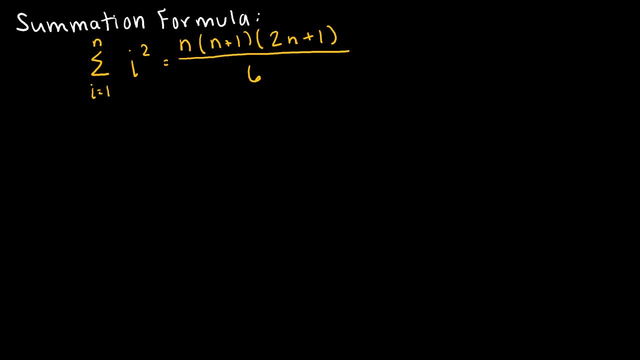 The next summation formula has to do with i squared. I'm not going to go through with you, like I did for the last formula, where this formula came from, just because it would take about 15 minutes and I don't want it to be that long of a video. But I do want to do one practice. 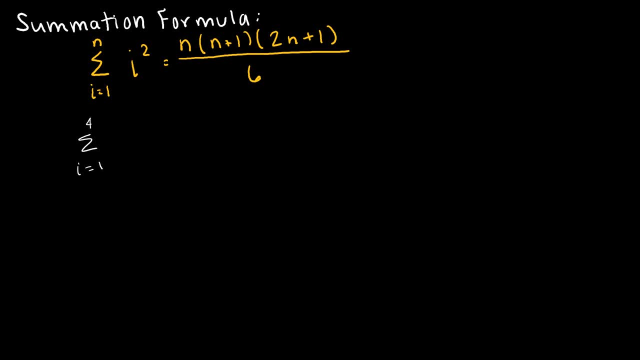 with you just to show you- not prove- that it works. this is not a proof, but just to show you that, yes, in fact, at least for 4, it works. So if I were going to do this by hand, this says start. 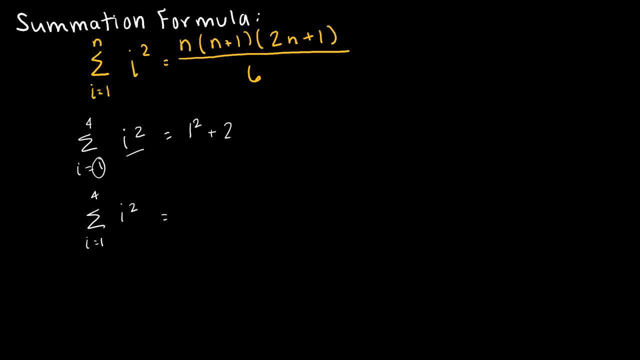 at 1, square it and then continue to increase until I get to 4.. So 1 squared plus 2, squared plus 2, squared, 3 squared plus 4, squared, which is 1 plus 4, plus 9 plus 16, which is 30.. So now I'm saying: let's. 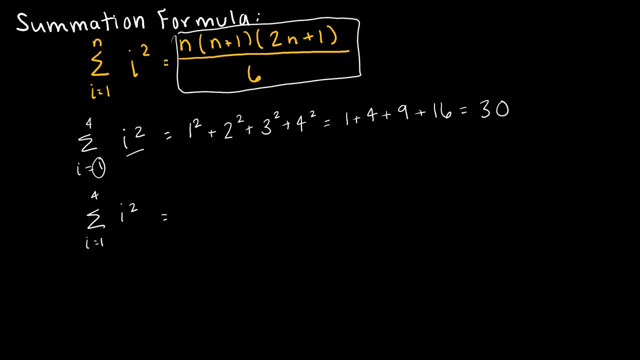 use this formula that says n times n plus 1, times 2n plus 1, divided by 6, should also give me 30. So n is 4, and then I'm going to take n plus 1,, which is 5, and then I'm going to take 2n plus 1,. 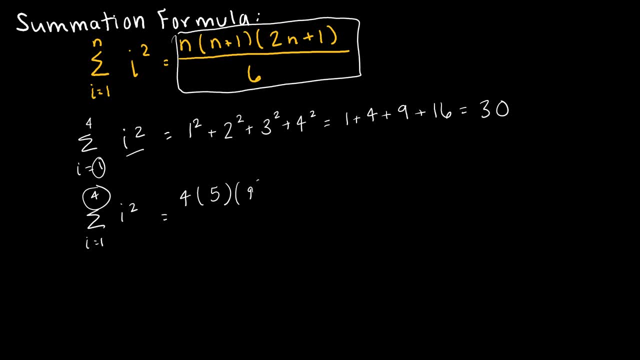 which is 2 times 4, or 8, plus 1,, which is 9.. And I'm going to take that product all divided by 6.. Well, 4 plus- I'm sorry- 4 times 5 is 20, times 9 is 180, and 180 divided by 6 does give me 30. 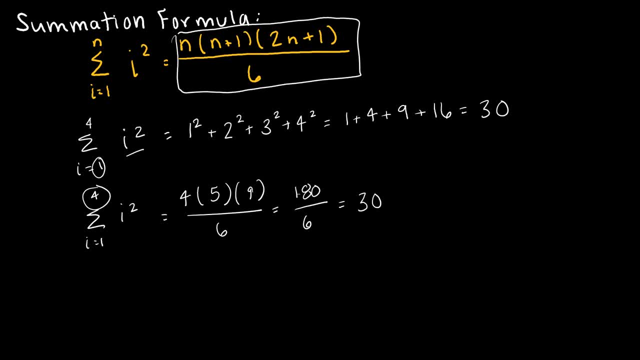 So we have verified that, at least for the value of 4, that this summation formula works. Now, before we move on, I do want to point out that, though these formulas are great for exactly what we did here, which is finding the sum, 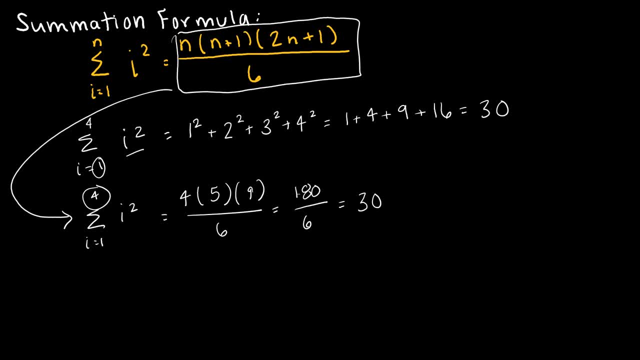 they're also great because when we're working on proofs and things of that nature, I am able to replace the summation as i goes from 1 to n of i squared with its equivalent counterpart n times n plus 1 times 2n plus 1 divided by 6.. 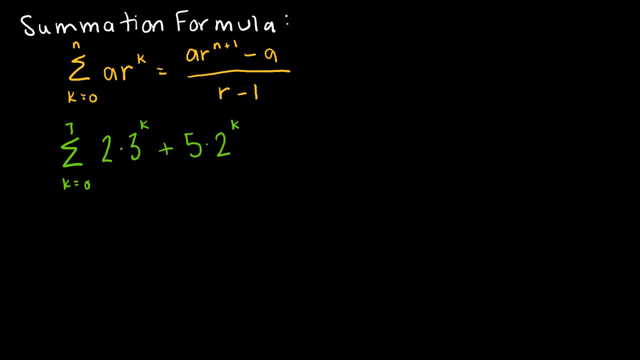 This is the last formula I'm going to go through with you, but just know that this is not an exhaustive list, So I just went through some of the big ones that will go that we'll use quite often in this course, and this one for sure is one that we'll use often. 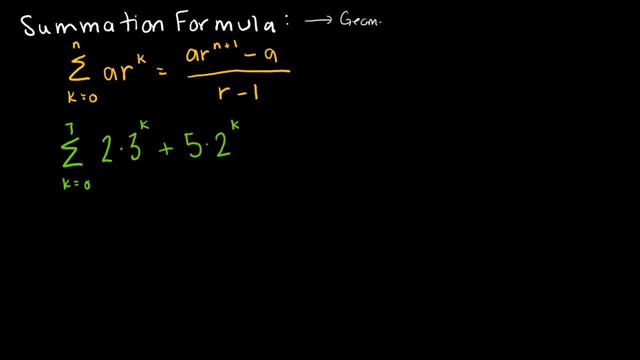 This is the summation formula for a geometric progression, or, as we called it earlier, just a geometric sequence. And just to refresh your memory, when we learned about geometric sequences, we said: to find a sub n, we're going to take a, which was our first value, our initial value. 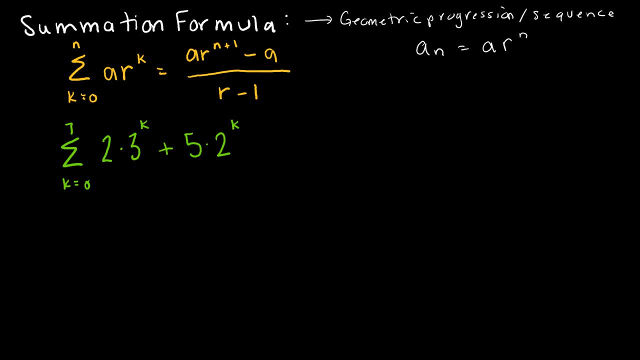 and we're going to multiply it by r to the nth power, And that's what a geometric sequence was all about. And, if you'll notice, that's what I'm doing is I'm finding the sum of the first n terms of a geometric sequence. 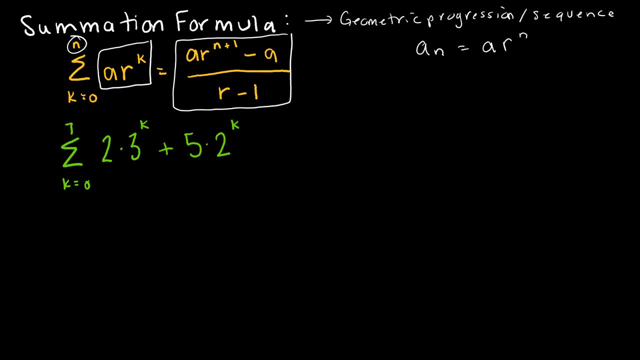 And according to the formula to do that, all I need to do is take a times r to the n plus 1, I'm going to subtract a and then I'm going to divide by r minus 1.. So I put an example here and I purposely made this example a little bit more difficult. 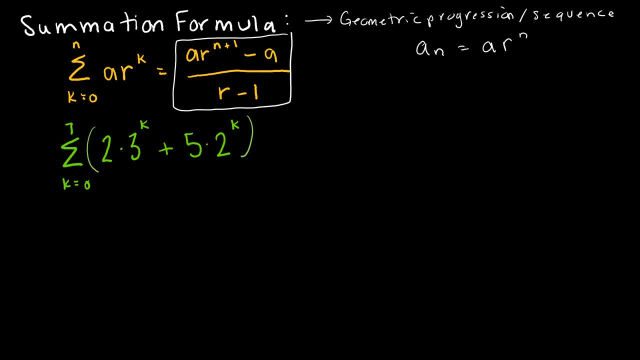 This should have parentheses around it. I made it a little bit more difficult because I wanted you to see the kinds of questions that you might get, And so we are going to use this new summation formula, but we're also going to use one of the properties that we learned in this video. 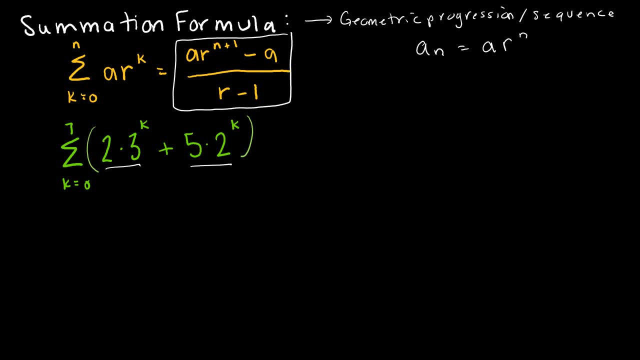 So, if you'll notice, I have the summation of essentially two different sequences, So all I'm going to do, then, is write this as the summation, as k goes from 0 to 7, of 2 times 3 to the k. 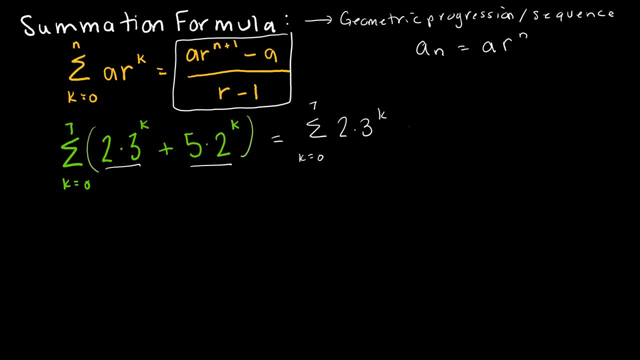 And then I'm going to switch colors so we have a different color to work with. plus the summation as k goes from 0 to 7 of 5 times 2 to the k. And again, that's just one of our properties that says if you have two different summations, 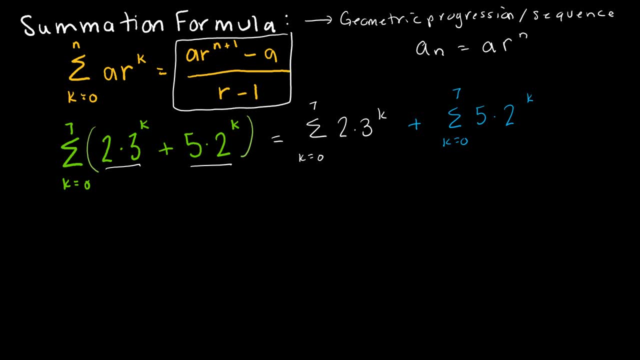 it's okay to break them up. Before I continue this question, one thing I do want to point out that I possibly didn't point out earlier is this: summation formula starts with k at 0.. Some of them start with k at 1.. 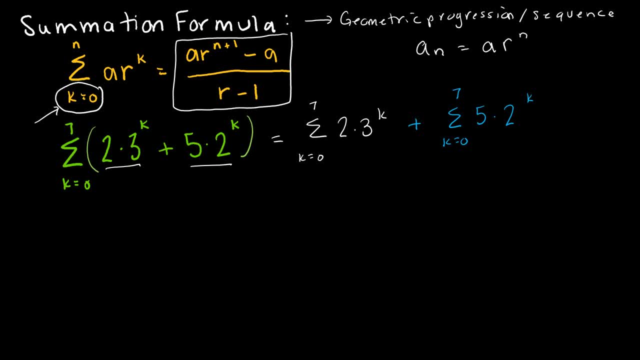 But when we went through the properties and I said, you might have to alter your sum to make it work- this is what I'm talking about. So if this one didn't start at 0, I might have to do some tinkering around with it, But thankfully we're not going to do that in this example. So now I'm going to. 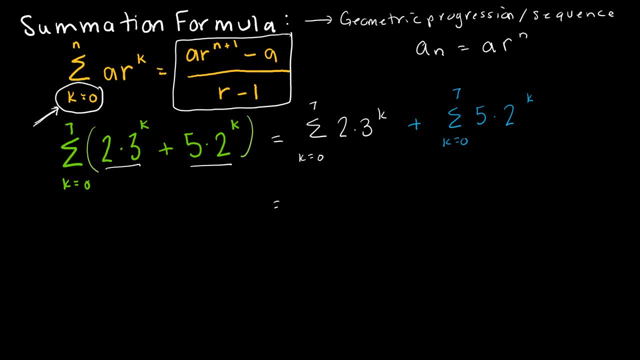 just use this formula. This formula, of course, a is 2 and r is 3.. So let's use the formula I have: k and a, which is 2, times 3 to the n plus 1, so n is 7,. so this is to the eighth power. 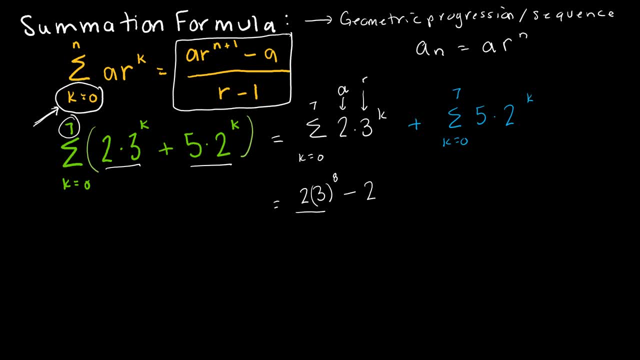 minus a, which is 2, and divided by r minus 1.. r was 3,, so 3 minus 1 is 2.. That's the first part. For my second summation, a is 4.. 5, r is 2,, and so I'm going to have a which is 5, times r, which is 2, to the n plus 1.. Again. 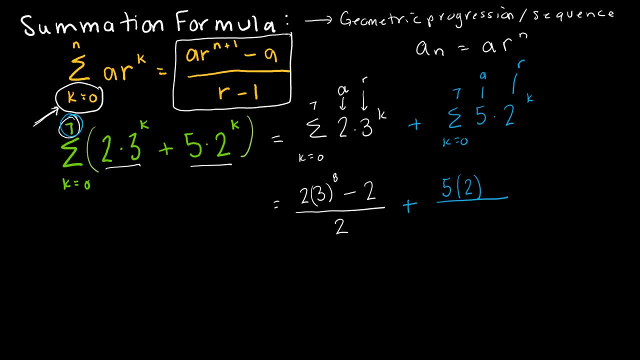 n is 7 from here. so 7 plus 1 is 8, and then minus a, which was 5,, and divide it by r minus 1, and r was 2,, so 2 minus 1 is 1.. So from here, I'm just going to use a calculator. 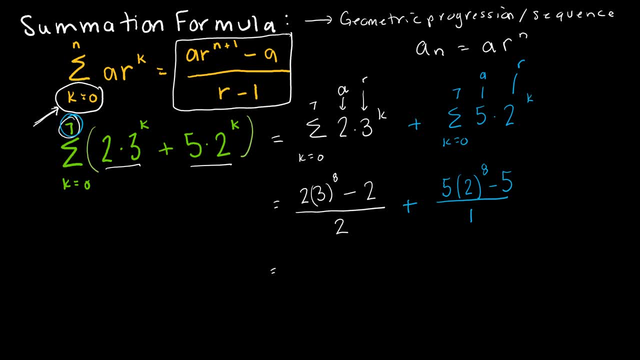 I'm going to take 2 times 3 to the 8th, subtract 2, this gives me 1, 3, 1, 2, 2, minus 2, over 2, which turns into 6,560.. Again, using a calculator, 5 times 2 to the. 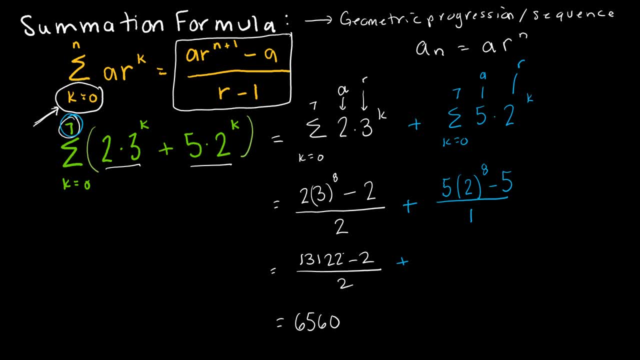 8th, subtract 2,. this gives me 1,, 3,, 1,, 2, 2, minus 2, over 2, which turns into 6,560.. 8 minus 5, over 2 minus 1, gives me 1,275, and when I add those values together, I end up with: 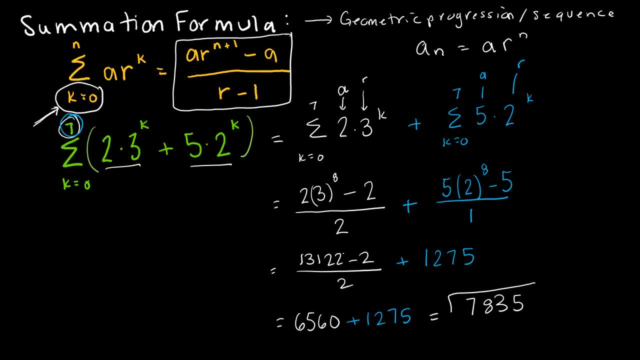 7,835.. Now, is this the only way I could find the summation of that? No, I could do this the long way, of course, and I could say what's the first value? 2 times 3 to the 0 would be 3 to the 0 is. 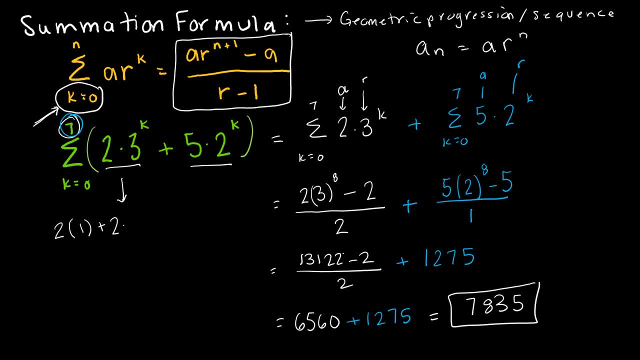 obviously 1, and I could say: what's the first value? 2 times 3 to the 0 would be. 2 times 3 to the 0 is obviously 1, and then 2 times 3 to the 1st, and then etc. and I'm not going to do it.